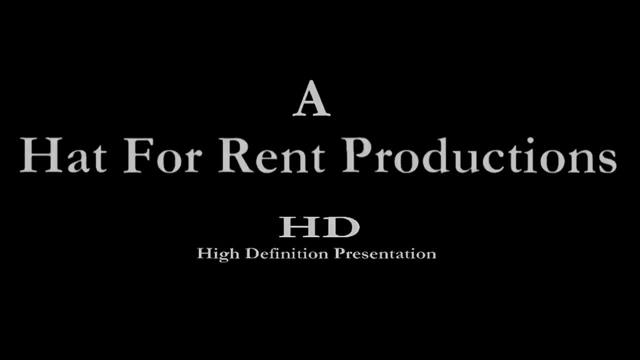 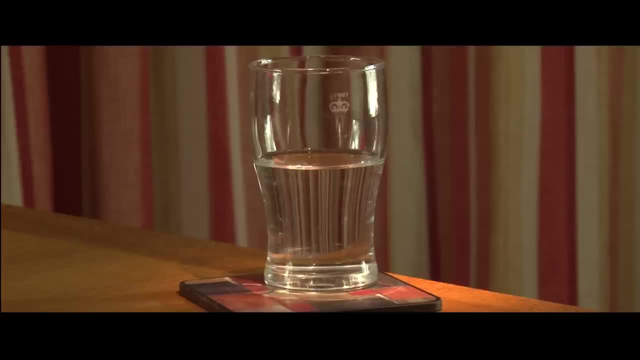 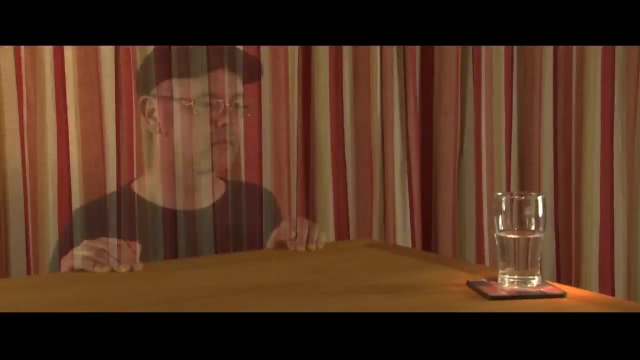 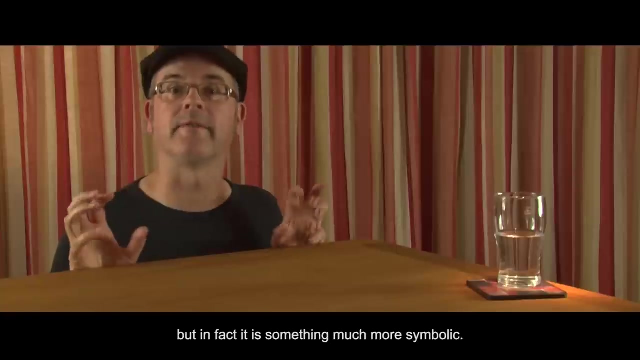 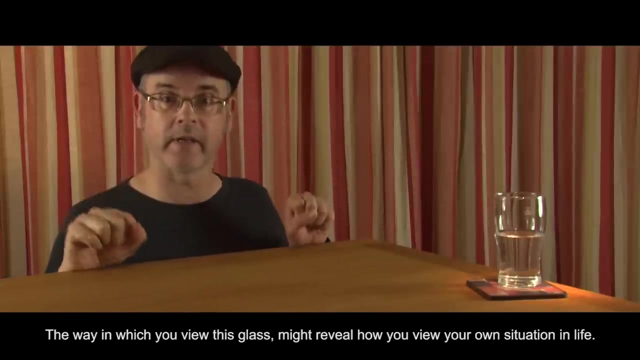 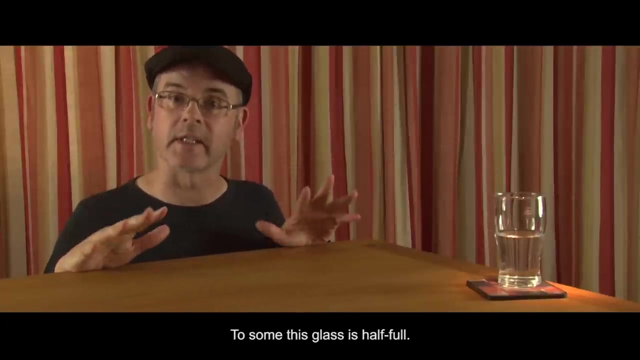 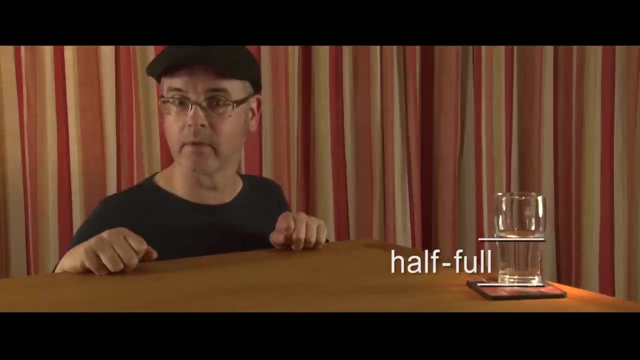 Thank you for watching of water, but in fact it is something much more symbolic. The way in which you view this glass might reveal how you view your own situation in life. Let me explain To some. this glass is half full. It is not empty. It still has something to offer you. There is still some water left in the 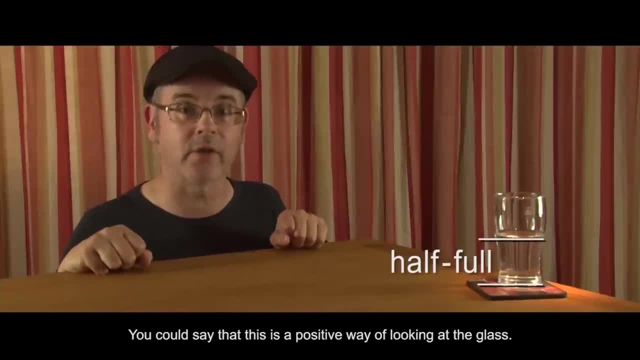 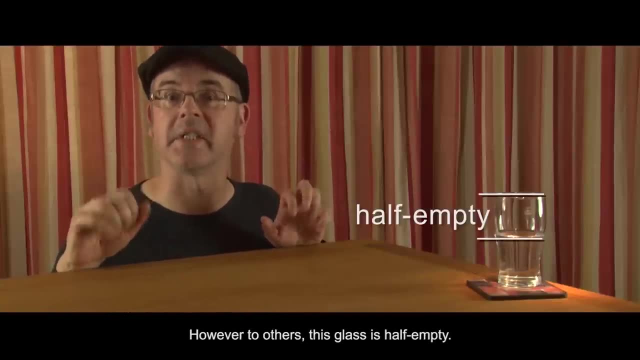 glass, You could say that this is a positive way of living, Looking at the glass. However, to others, this glass is half empty. There is not as much water in the glass as there could be. This could be viewed as being negative and pessimistic. 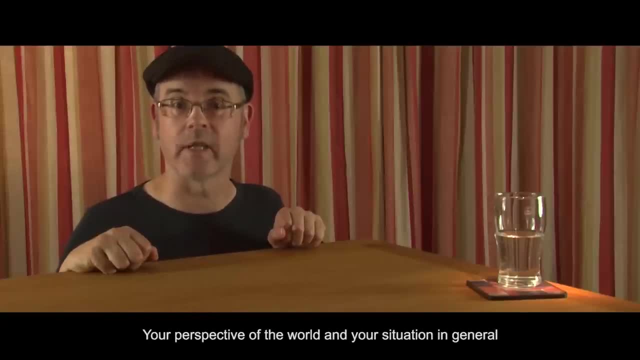 Your perspective of the world and your situation in general can often be judged by whether you see the glass is half full or half empty. As for me, well, what do you think? Is my glass half full or half empty? Being able to see the bright side of something is not easy, But it can be done. After all, tomorrow. 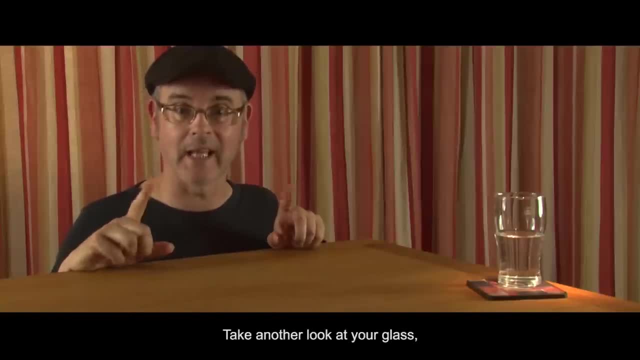 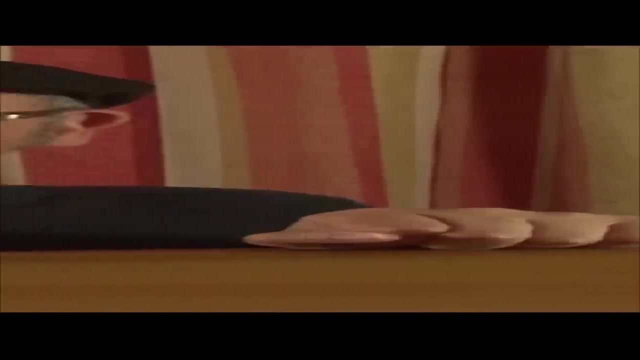 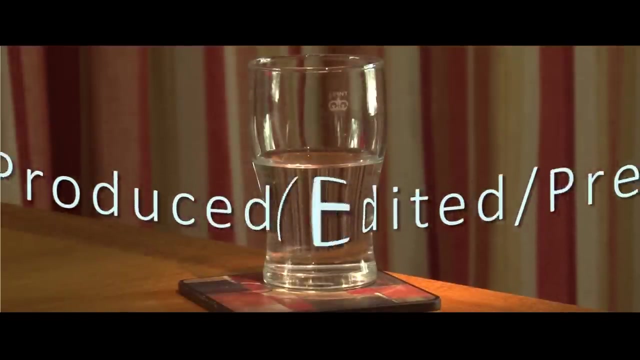 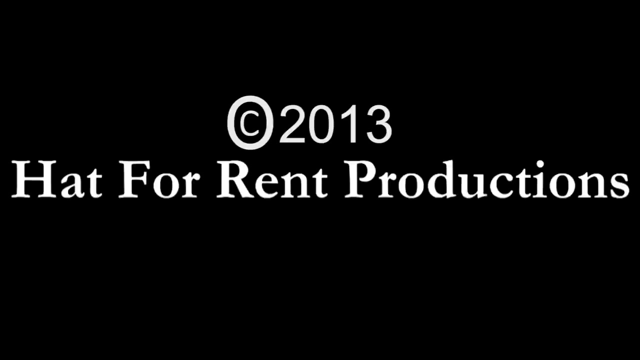 is indeed another day. Take another look at your glass. You might be pleasantly surprised by what you see. This is Mr Duncan in England saying thank you for watching me teaching you And, of course, ta-ta for now. Thank you for watching.